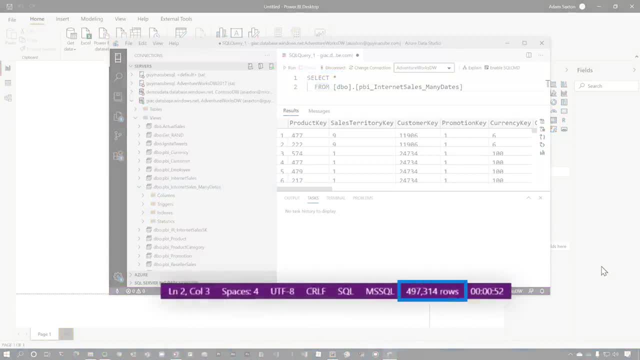 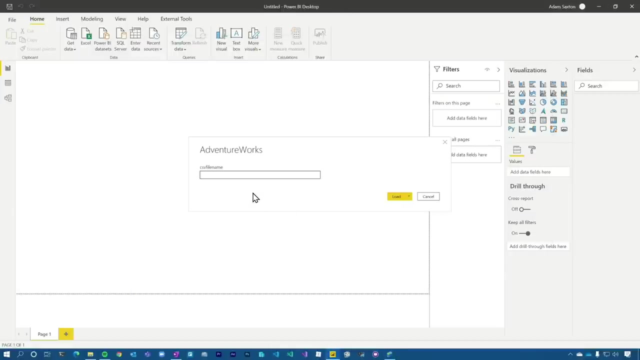 right At the bottom of this, you can see 497,314 rows, And right next to that you'll see 52 seconds it took to execute this query. right? That's our baseline. It took 52 seconds to grab this data. So now I've created a Power BI desktop file. It's a template file, So I want to get a. 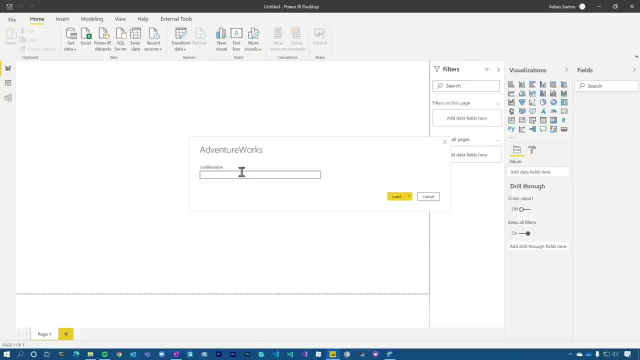 clean record of this query And I'm going to go ahead and do that. So I'm going to go ahead and clean slate, bring in that data and see how long this is actually going to take. So I'll add in my parameter and then let's hit load. 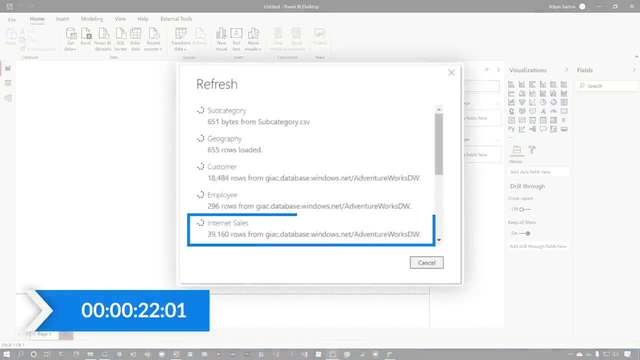 What I want you to do is pay attention to this internet sales where it says loading data to the model right, Because this is the same. this is not the internet sales two, this is internet sales, All right. So that's done: 497,314 rows, And if we look down here, we've got a lot of data. 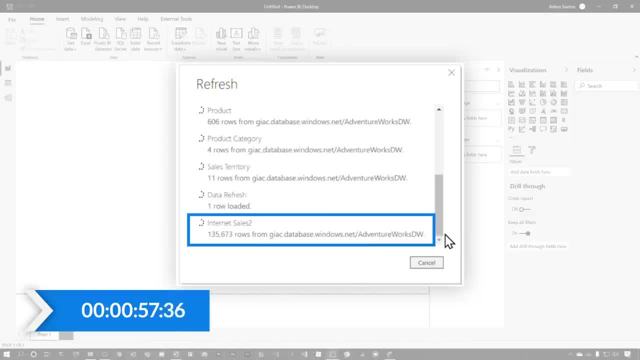 down here. internet sales. two taken longer. What's going on? Why'd the other one return fast And this one's taking a little bit longer to run? Now it's done with that data, but now it's still taking some time to run. 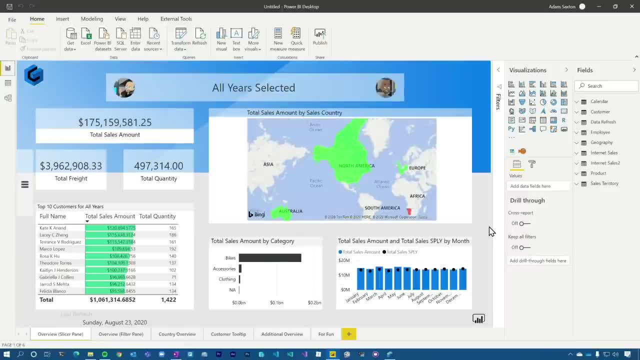 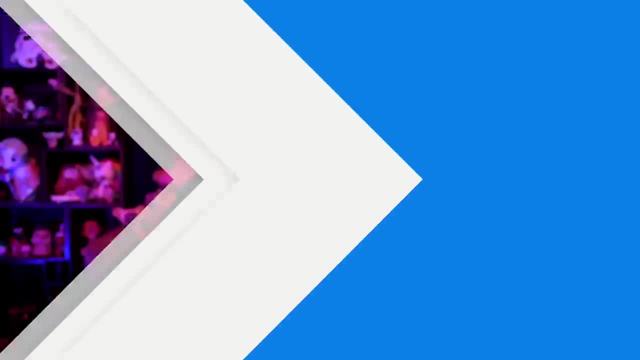 And then bam, we're in All right. So let's break this down a little bit. We're going to go to power query. There's a couple of things to realize As part of this. first thing to consider here is your actual data source performance, right? So? 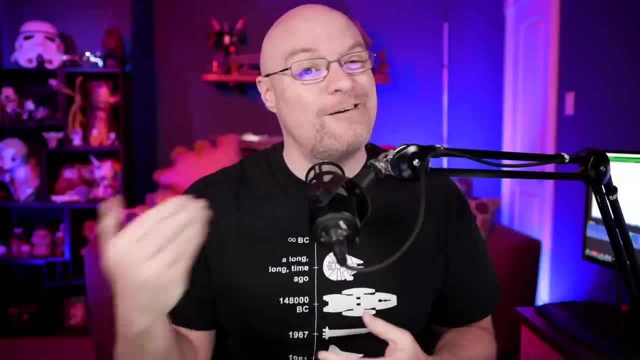 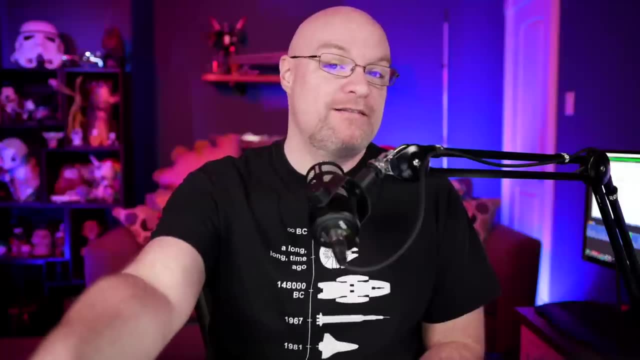 say it's SQL server, If you're issuing a query, how long does that take to come back? That's the first thing I do when I break this down. let's get a trace, Let's actually see the queries that power BI is issuing. How long does that take to respond? And then maybe there's some tuning you. 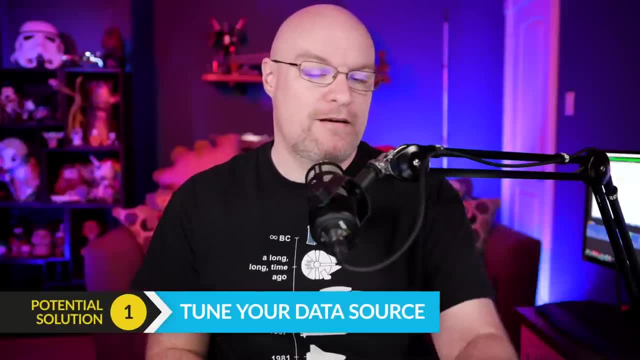 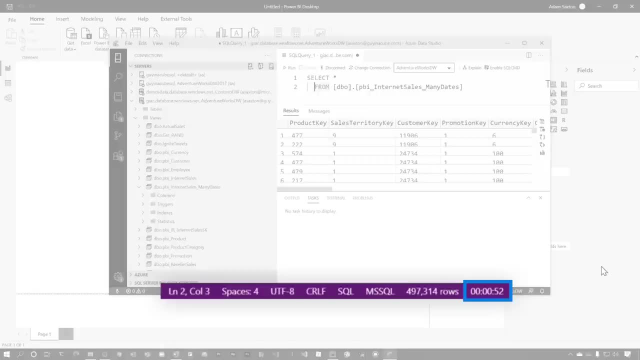 can go do on your data source side. So that's the first potential bottleneck. That is your data source In this case. we know that when we just issue that select star, it comes back in 52 seconds for that particular table. That's our baseline. 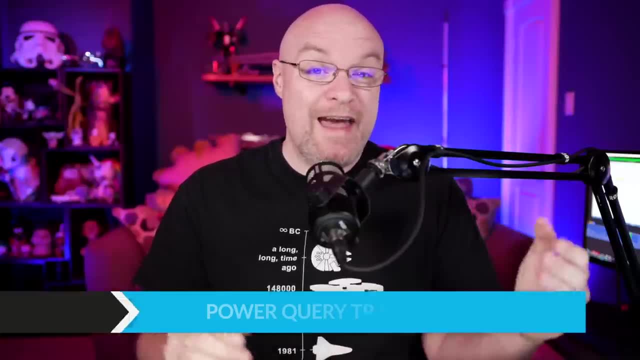 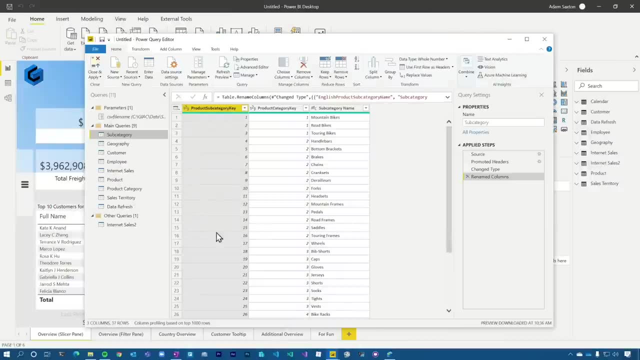 So now that we know the data source, let's move on to the second piece of that, And that is the actual power query transformations and what you're doing from that standpoint. So what do I mean by that? The power query transformations and whatnot. If we go look at internet sales too and we go to 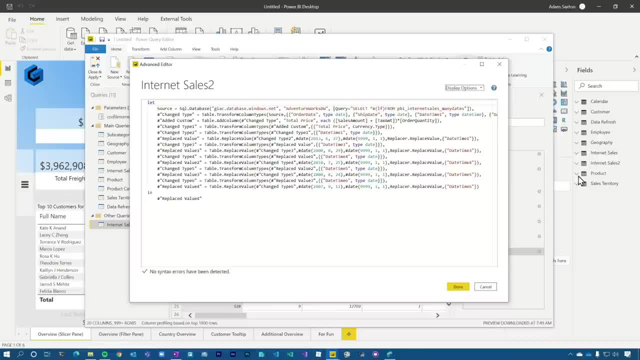 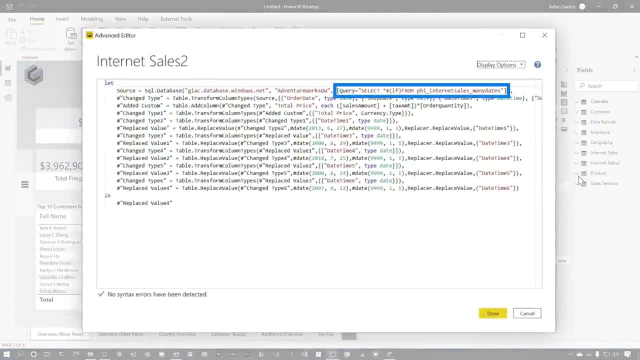 advanced. there's a couple of things that are a potential warning sign here. The first: here we're going to see query equals, select star and the actual item. This is what's referred to as a native query, or you're actually supplying the SQL query, that's. 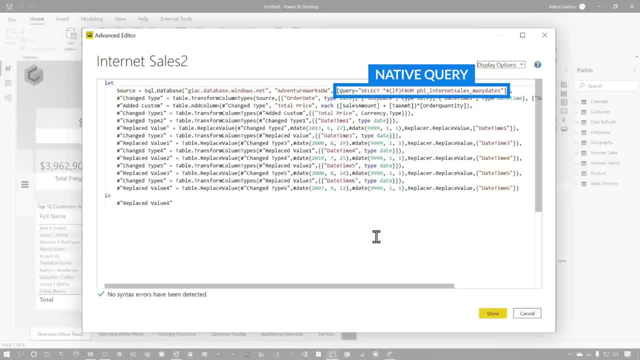 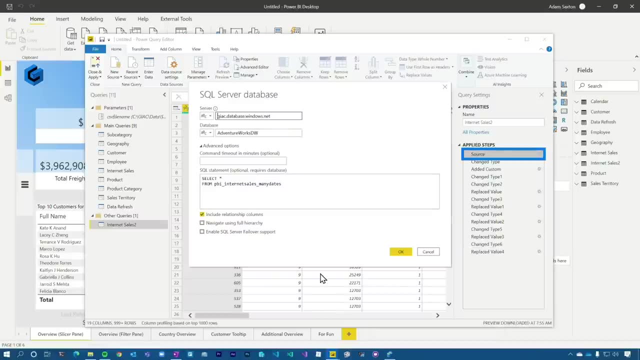 going to be issued to the data source. Now, this is the M syntax, so it looks a little scary. Let me actually go click on the source- the gear next to the source. You can see this. So when we're connecting to something like SQL server or like another relational database, 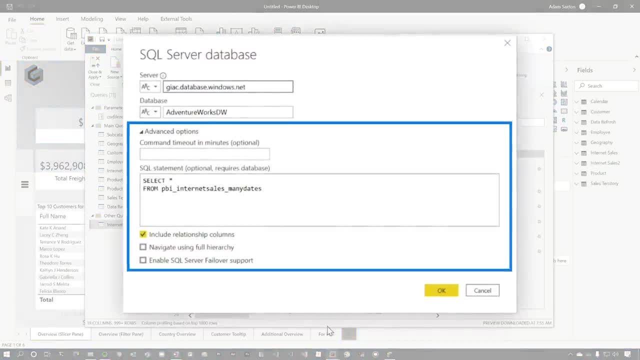 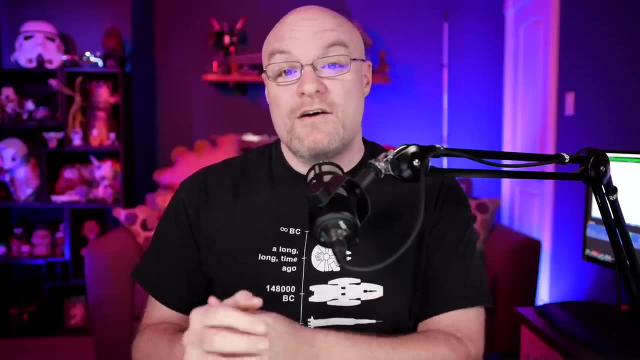 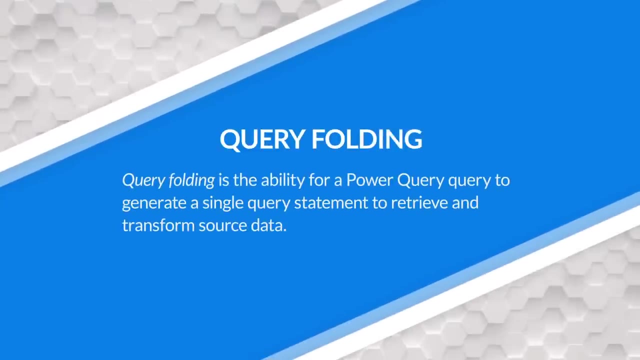 if you expand this advanced options area, you'll see the SQL statement where you can supply your own query, That is, native query. This blocks what's referred to as query folding, And so the idea of query folding- a term I coined in one of our live streams- is, think about it like query squishing. So if I've out, if I have all of, 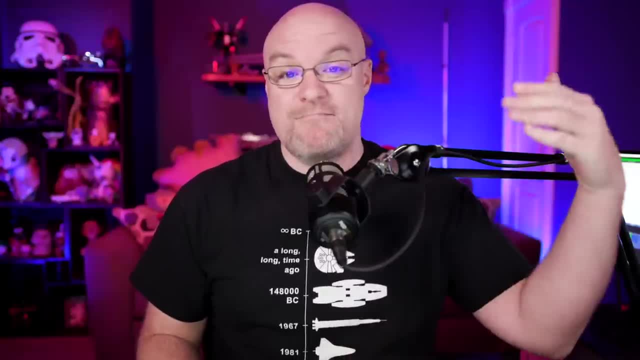 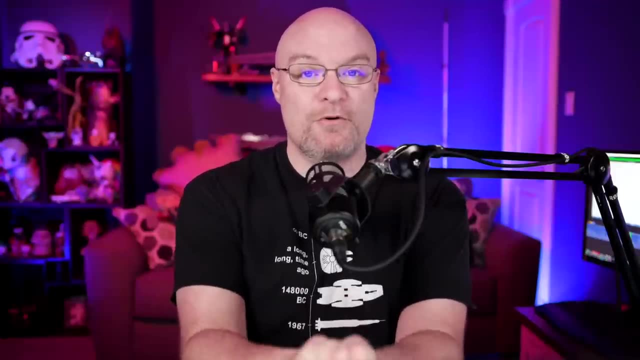 these transformations- like maybe I'm renaming columns, I'm removing columns, I'm doing a calculated column of some kind- Those get written into the SQL query That's going to go back to the data source When I issue this native query. that doesn't happen. 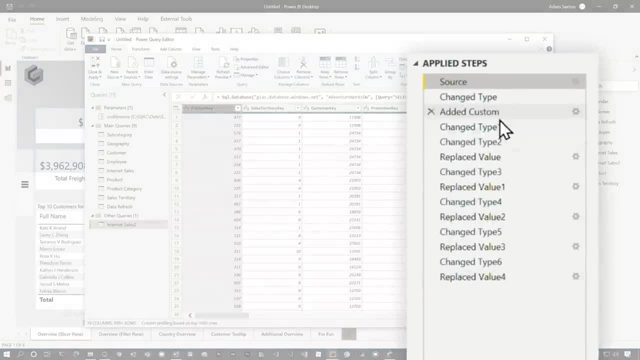 So let's go back to the SQL query, Let's go back and look and we can see here that in our applied steps we've got our query, which is the source, And then we're doing all of these items: I'm changing types, I'm replacing values, 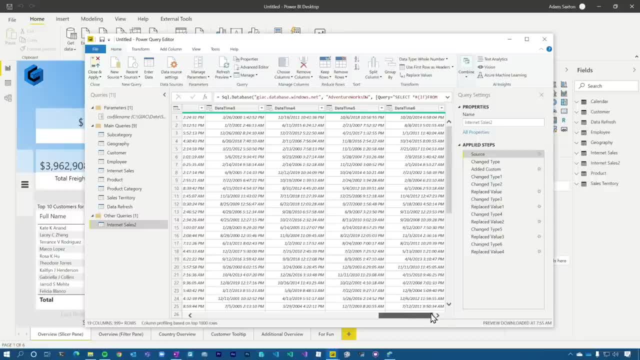 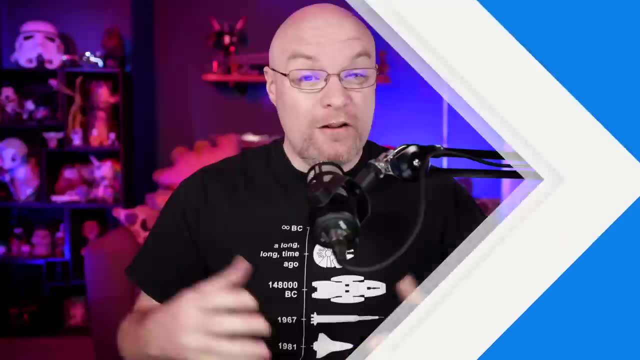 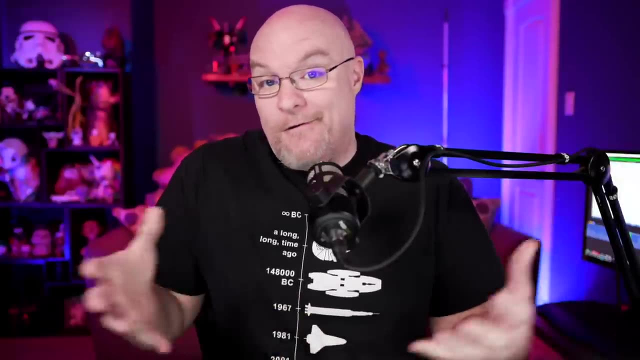 And I actually also created- or maybe not in this one, but if you create a calculated column, that will also take play in this. All of these transformations happen after we execute that, so that's something to consider: for how long something is. 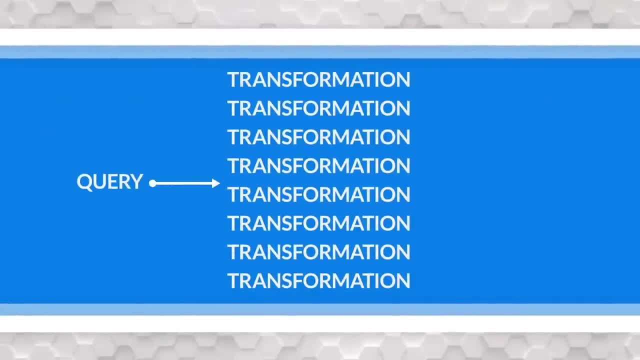 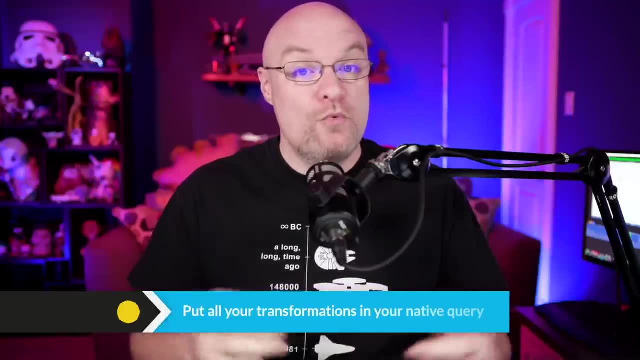 So the more transformations you do after that native query, that's adding overhead to what you're actually trying to do. Typically, what I recommend is: if you are going to use a native query, you want to do everything. all of your transformations in that SQL statement pushes you. 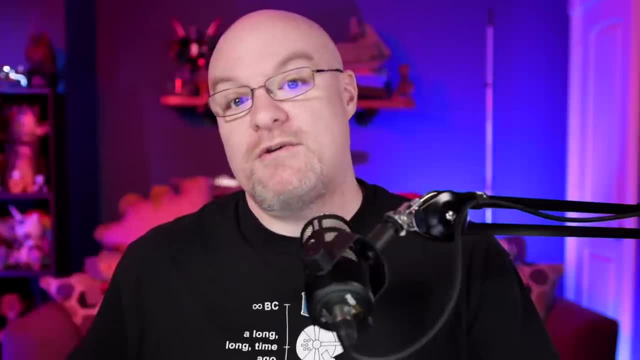 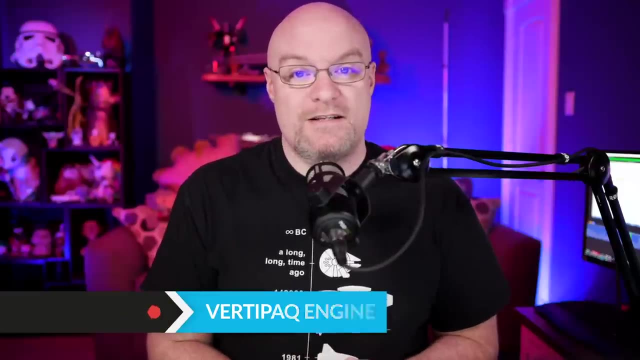 need to manually push it back to the source. try to avoid doing transformations after the fact. The third bottleneck is going to be what actually happens in the VertaPack engine itself. So we're getting all of that data and we want to put it into your old query. 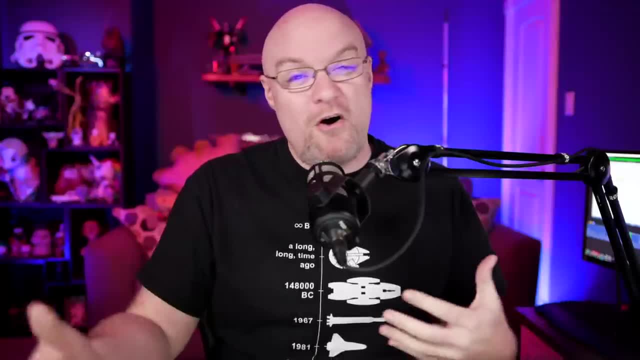 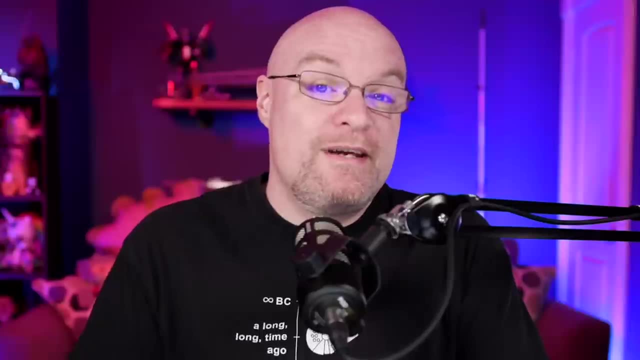 to the data model. So the VertiPaq engine is gonna come into play. It's gonna do all of its crazy stuff with compression and sorting and whatnot, But the thing to realize here is if you're doing any type of calculated columns or calculated tables, 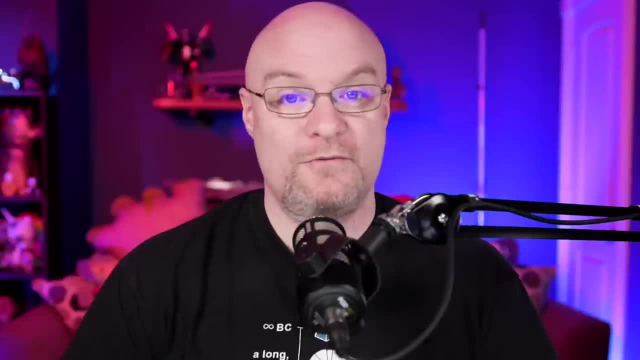 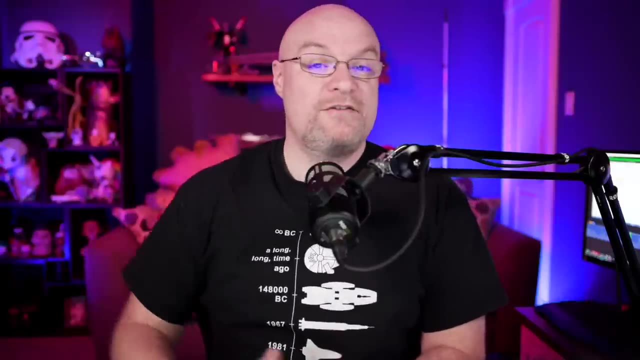 those happen after all of the regular table with, like what you're getting from your power query. it all happens after that, So that can add additional time onto your refresh. Let me show you a good example of this. What I'm gonna do here is I'm just gonna enter. 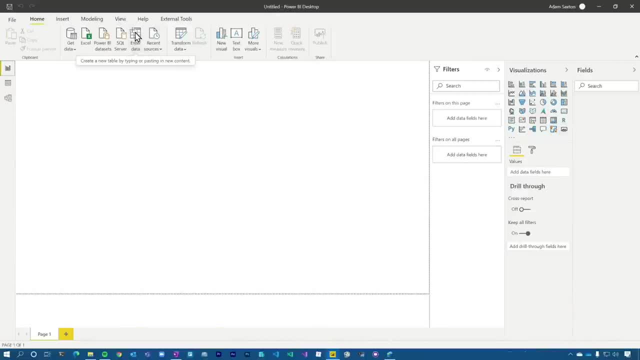 some data And, if you remember, in a previous video I had where I looked at like auto date time and how that can really bloat your actual model size. I'm gonna actually do that again here, just to illustrate what this is doing. Okay, so what I've got here is I have a date table. 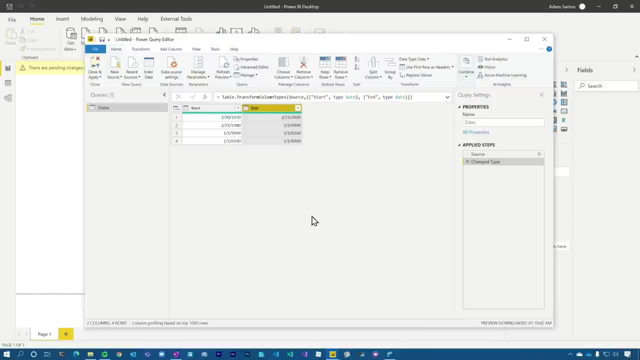 and I've got two columns here, start and end, with four rows right, One table, two columns, four rows that I manually entered the data, So there's not even a data source that we're going out to, So I don't even have to worry. 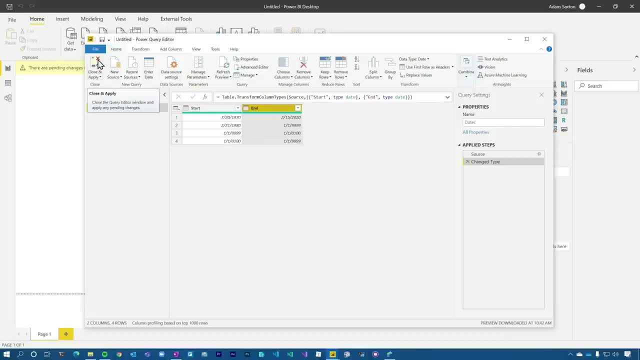 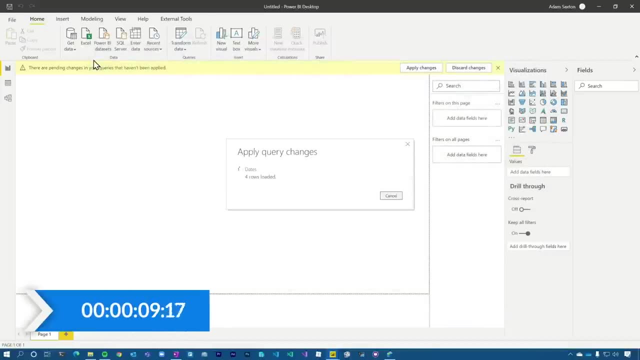 about the data source performance. So let's hit close and apply and see how long this is going to take- Four rows, And I'm not gonna cut any of this, so you can actually see that this is gonna take a while. What it's actually doing is building out. 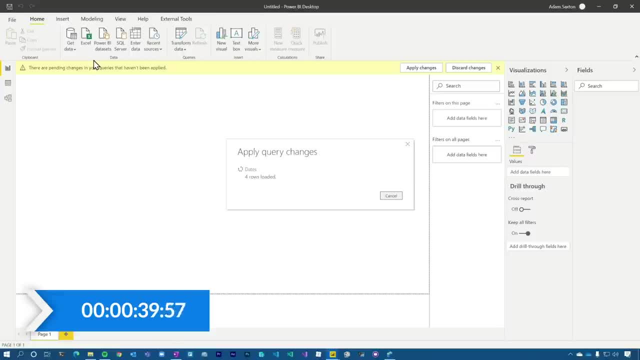 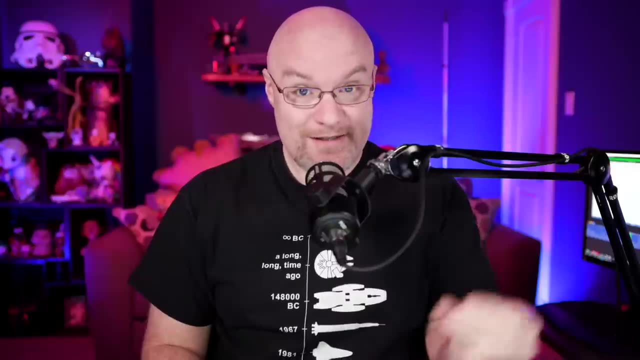 this a calculated table that's getting generated for both of those two columns. That's that large local date table And then bam, we're up. That took a while. It wasn't like insanely fast, but that's because it had to build out. 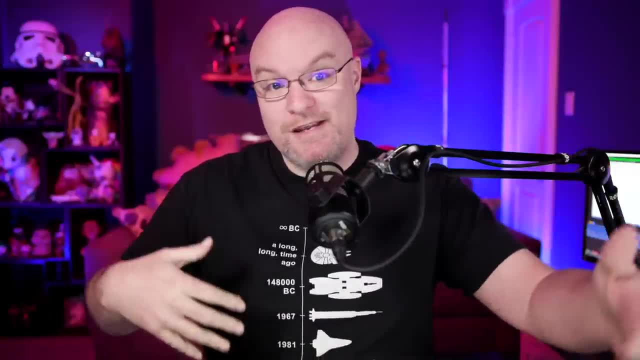 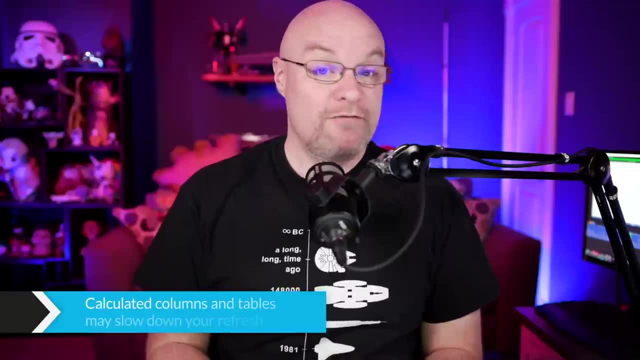 those two calculated tables that have like three plus million rows in each one. It's gotta build that out. That's gonna take time. So that's another thing to consider is if you're doing a lot of calculated columns or calculated tables, that is added overhead. 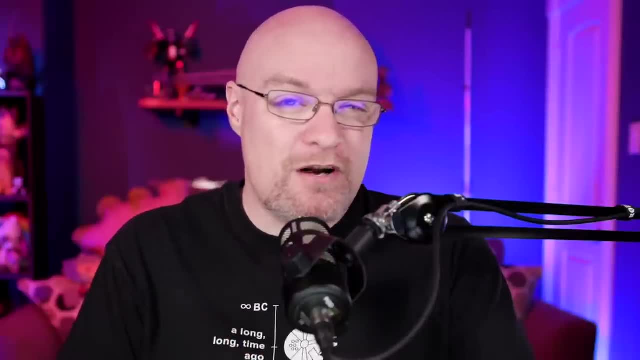 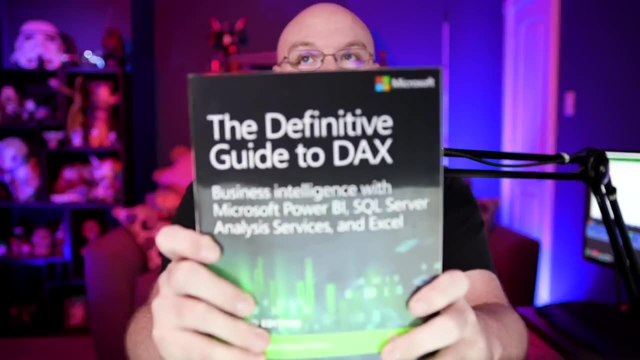 There's other factors there, too, and it relates to the structure of your data. So one thing I would definitely recommend you do is pick up something like this, Like this book here- Definitive Guide to DAX- And I'll have a link in the description below.